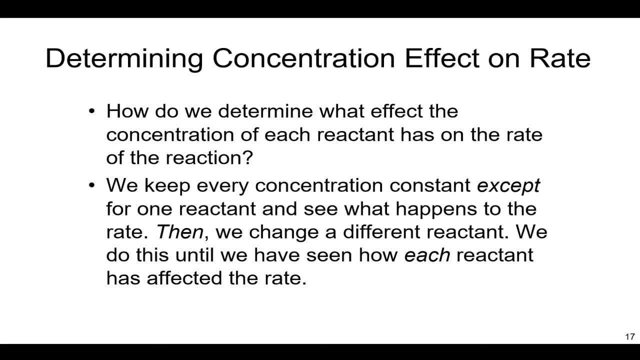 we determine what affects the concentration of each reactant, How that affects the rate of the reaction. So the rate of the reaction is the speed of the reaction. that is sort of the fundamentals of kinetics: how fast does a reaction occur? But we know that concentration will affect. 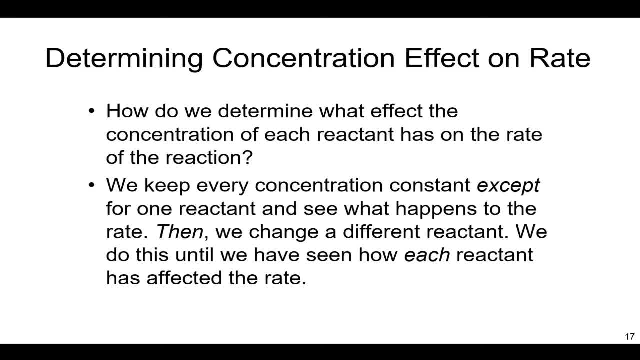 said reaction, And in the previous lecture we saw that borne out in tables and graphs and data. but it's actually more complicated. We know that reactant concentration affects the rate, but it is a one-to-one ratio. Is it a squared ratio? Is it, you know, logarithmic? What is the? 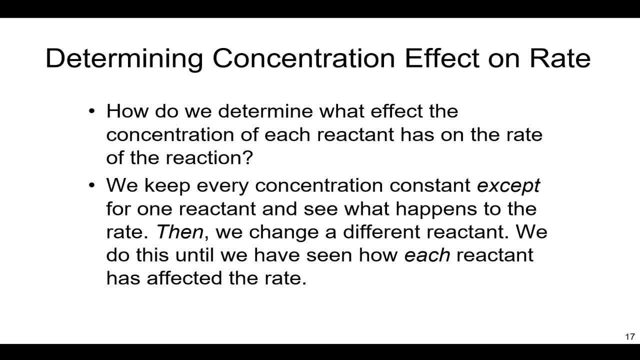 quantitative rate. What is the rate of the reaction? What is the rate of the reaction? What is the quantitative relationship And how do we determine that experimentally? So that's what we're going to talk about today, by introducing the concept of a rate law. So that's what this 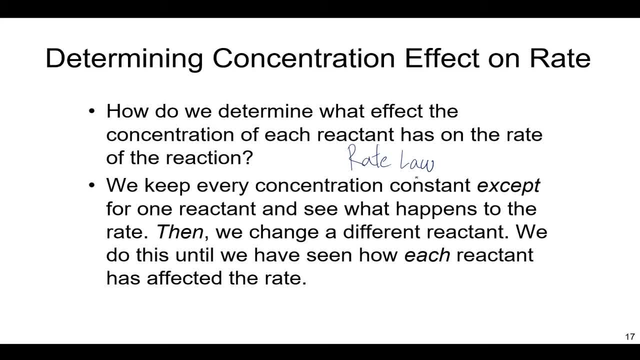 lecture is primarily about The way we do this in an experiment, and all of kinetics is really driven by experimentation. you then build the theories of the reaction mechanisms from the experiments we're going to talk about today, And the way we do this is by keeping the concentration. 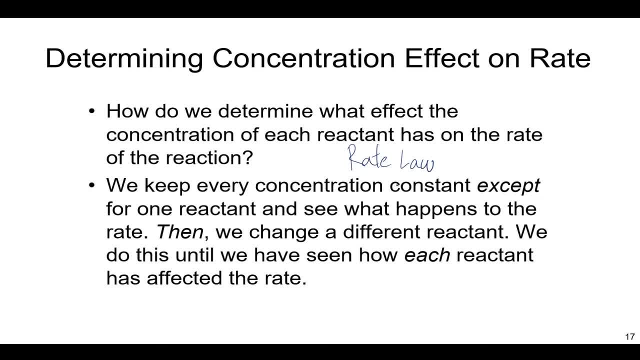 of everything constant except for one reactant, and see what happens to the overall reaction, so that we tease that out. And then we're going to talk about the concept of a rate law that specific reactants affect. So if you have A plus B plus C goes to D. well, first you hold B and 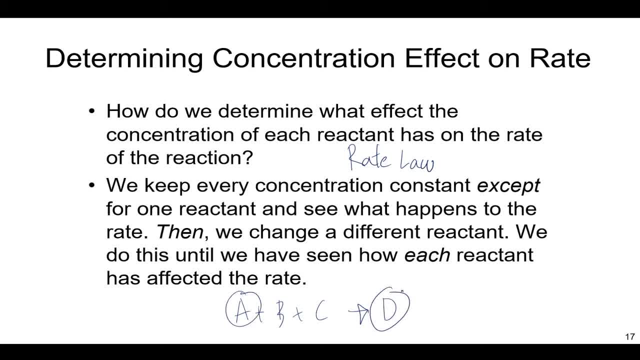 C constant and change A and see what effect it has on D. right, Is it a one-to-one ratio? Then you hold A and C constant and change B. Maybe you double B and D goes up by a factor of four and there's sort of a squared relationship between them, et cetera, et cetera. So that's. 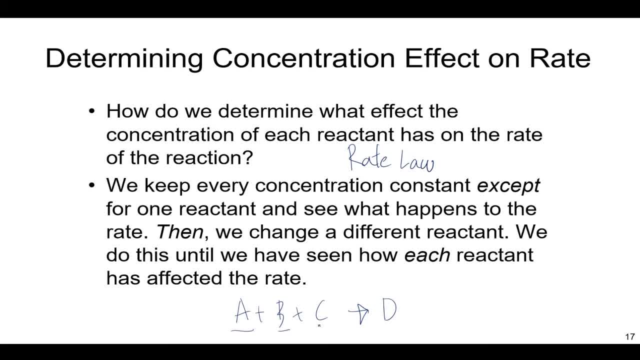 how we do it? experimentally, We move through reactant A, then B, then C, holding the other two constants constant and seeing what effect it has on the overall conversion from reactants to products. Now let's look at this in some tabulated data. 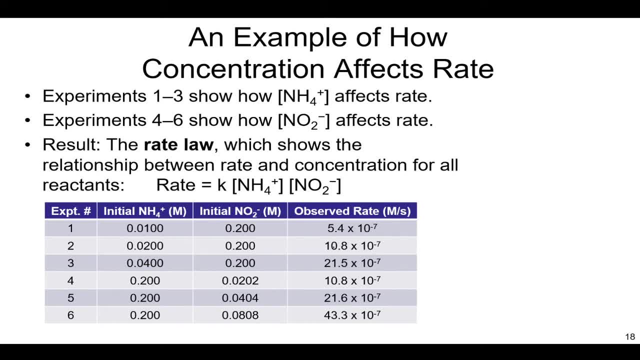 for a given reaction shown here where we're really converting this ammonium ion and this nitrogen dioxide ion into some products. What the specific products are aren't really important for the rate of the reaction. We know we can express the rate, as we learned last lecture from I. 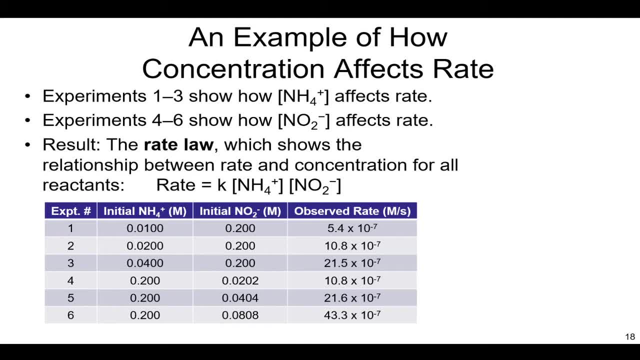 reactants or products. Here we're just looking at reactants. Now the rate law overall shows the relationship between the overall rate and the concentration of reactants, And this is something really important. The rate law, okay, is always going to look something like this, but it's always 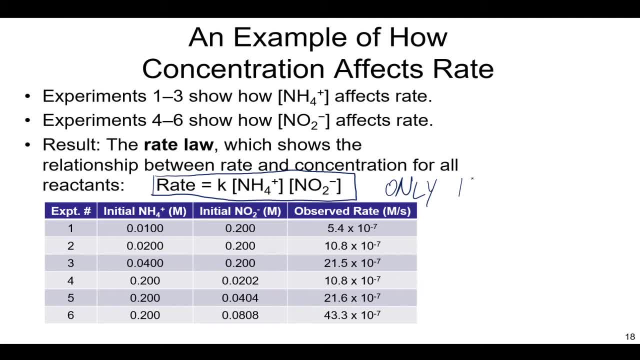 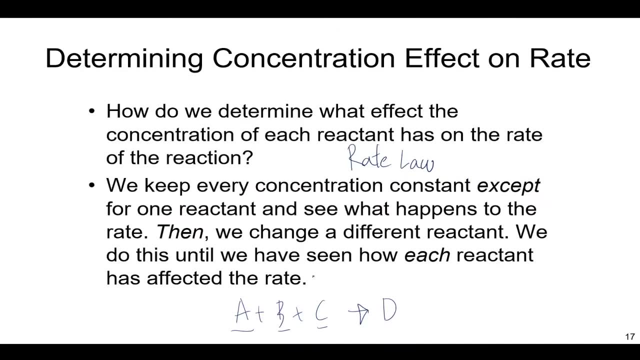 only in terms of the reactants. So in analogy to this reaction shown here, the rate law could be equal to something with A and something with B and something with C, but D will never appear in this rate law. okay, And the reason? 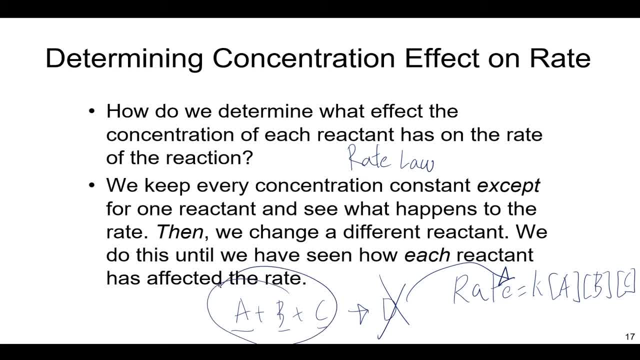 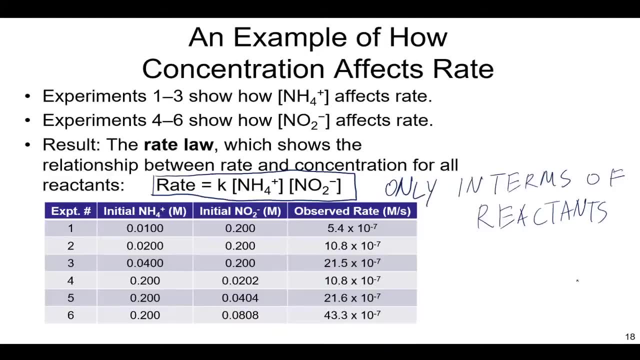 is, we're setting up a reaction by mixing A, B and C together and letting it go, And we want to know how the rate of that reaction proceeds based on those concentrations that we've set up. Okay, so the rate law is only dependent on the reactants here. Never list a product in the rate. 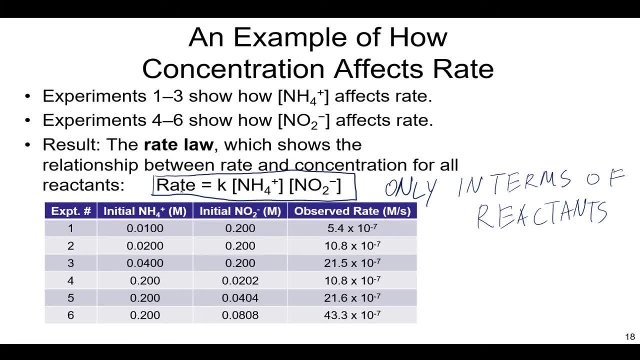 law. okay, This is the quantitative relationship between this rate and the concentration of all the reactants, And we'll get to this. but there can be powers up here like twos, threes, some integers, or there can be a one which is implied, or it can be to zero, which means it doesn't really. 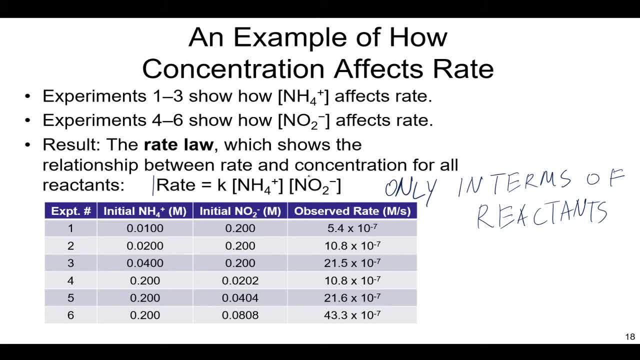 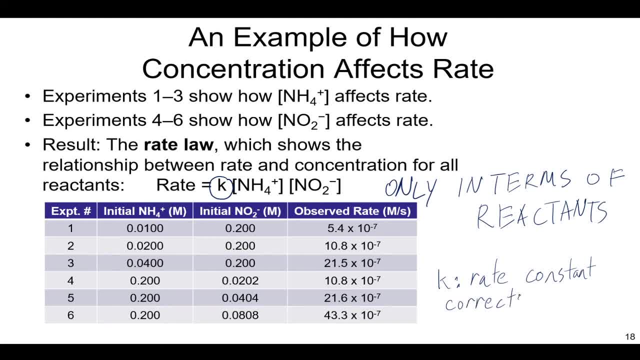 And it sort of encodes or has the temperature dependence of the reaction built into it And we'll see that in future lectures We'll learn about Arrhenius and his great contributions to chemical kinetics, But this K you'll see in all rate. 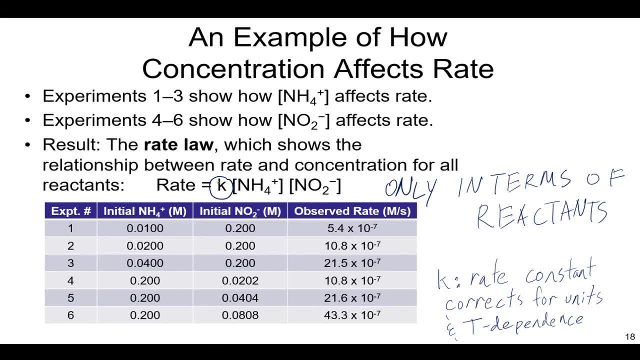 constant equations. So let's look at this, So let's look at this, So let's look at this. So rate laws, i should say, and it's just a rate constant, it's a constant only at that certain temperature. right at different temperatures there are different rate constants. but it also corrects. 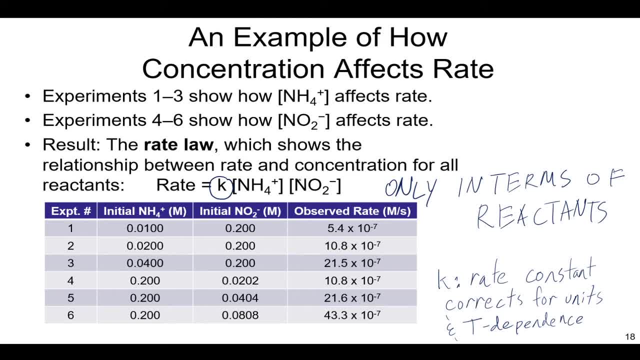 for the units now the rate law we use to determine reaction order as well, and we'll see that in the coming slides. so imagine we have this sort of data like this for nh4 plus and no2 minus, and we'll actually do the math on this to extrapolate, uh, how we come up with this overall rate law from this. 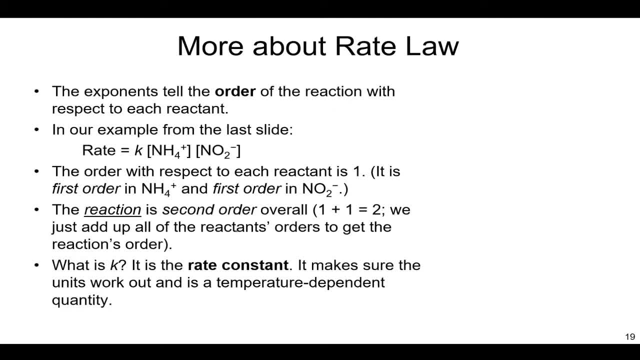 data. but first just going through sort of uh, each part of the rate law in a little bit more uh detail. the exponents tell us the order. so some vocabulary, vocabulary we need to know here for the rate laws the exponents are the order. so i'm going to write a general rate law that you could see. 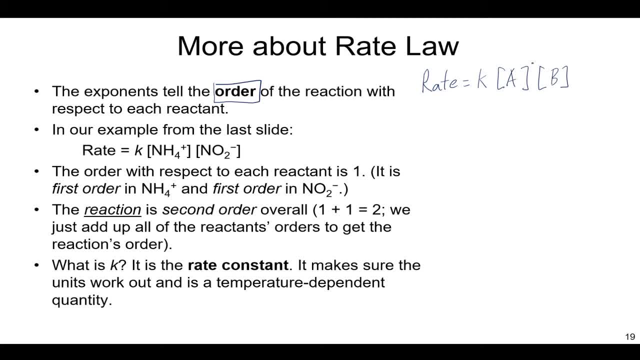 for a reaction. okay, now, this is not exactly typical, but i just want to show an example. okay, the reaction here is a plus b goes to c. now this overall reaction you might think, means a and b. the dependence on how fast this happens is a one-to-one ratio, because the coefficients, the stoichiometry, is one to one. okay, but that's. 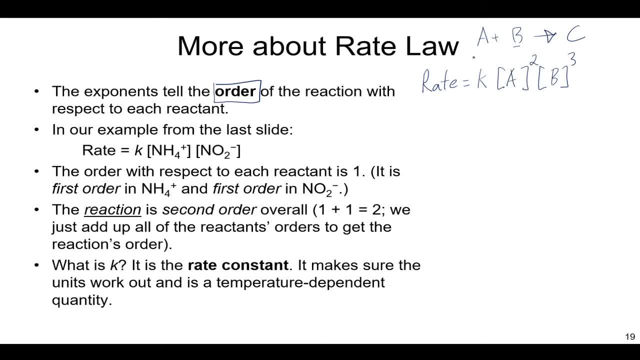 absolutely wrong. that's not the way kinetics works. okay, the overall reaction is more a balance of where do you start and where do you finish, but it doesn't tell you exactly what's happening at the molecular level. yeah, we talked about this in the previous lecture. feel free to go back and watch. 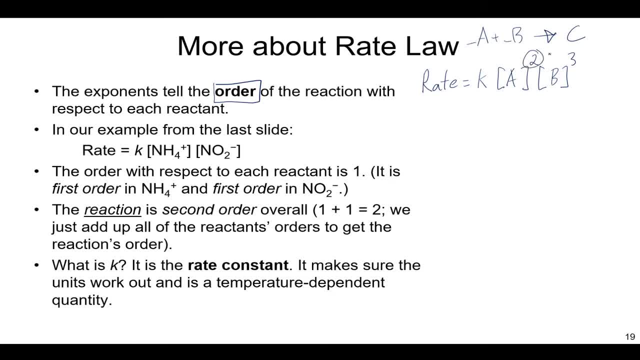 that video. you can't just take these coefficients and make them the exponents. that is a very, very common thing for students to do and that will get you zero points. okay, these have to be determined experimentally and these exponents tell us the order of the reactant, of the reaction. 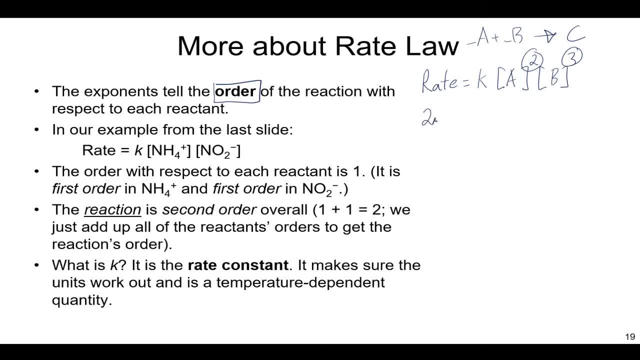 with respect to each reactant. so this would be second order with respect to a and third order with respect to b. right the exponent tells you the order with respect to it. overall, it is fifth order, adding up the exponents. so this is just some vocabulary we need to learn. 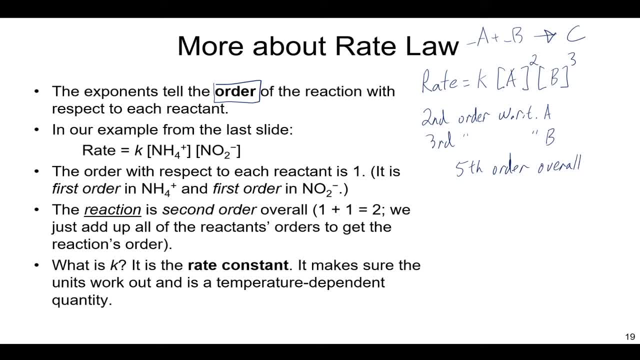 right, and this order tells us something about- as we'll see in future lectures- the molecularity which means how many of these things need to bump into each other for a reaction to occur. so this complicated rate law actually, as i said, is not typical, but it suggests something about two a: 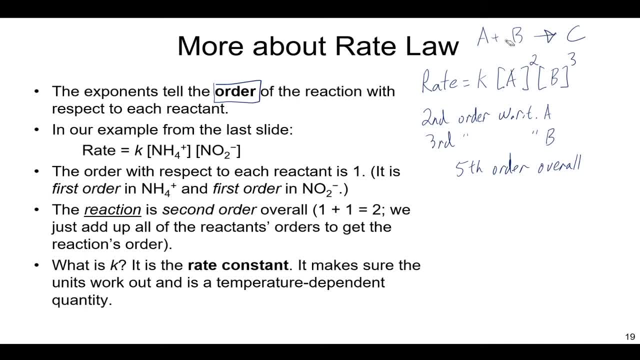 molecules having to bounce together, right? the overall reaction here suggests a bounces into b and makes c, but that's wrong. okay, chemists have got their heads. it's either b or h. rather cos Esteban, in my 해�lure maher the Flame. другие equations possible. mı şey raGEks них a etcao père. 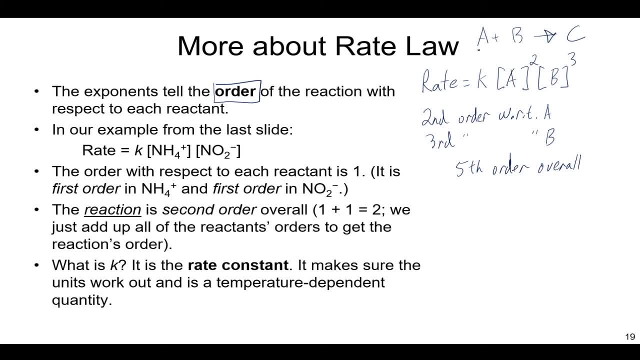 but the overall reaction here suggests a bounces into b and makes c. but that's wrong. okay, chemical reaction, koştak e to design la milk chemists write these things out for where the thing starts and where the thing ends. it doesn't tell you how many things bounce into each other to create the products. and that's really the level. 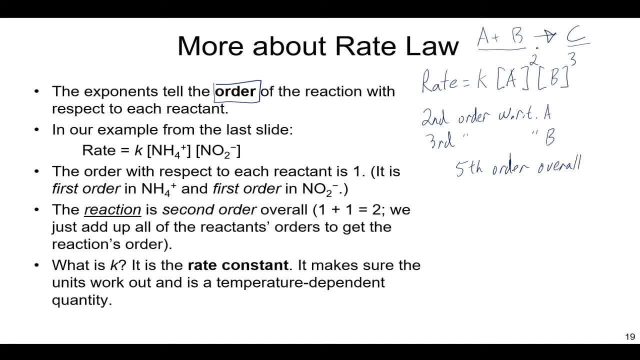 of detail. we need to know to figure out how to make a drug to block that process or make a catalyst to encourage that reaction to occur, if we're trying to remove certain pollutants from our cars, for example, so we need to know the reaction order to find out something about the. 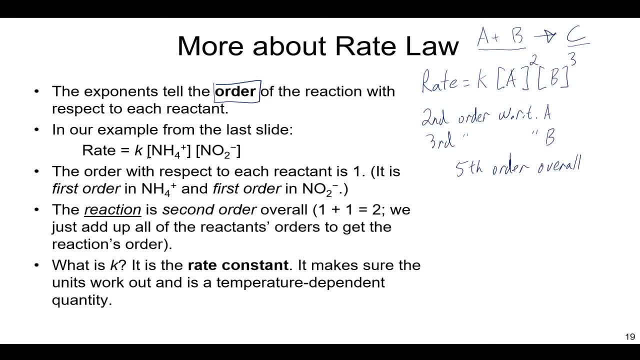 mechanism. now on the example from the last slide here, if this was our rate law, we would say: well, the one is implied here for each of these, and that this is first order with respect to ammonium and first order with respect to nitrogen dioxide ion. it's second order overall, just adding up these. 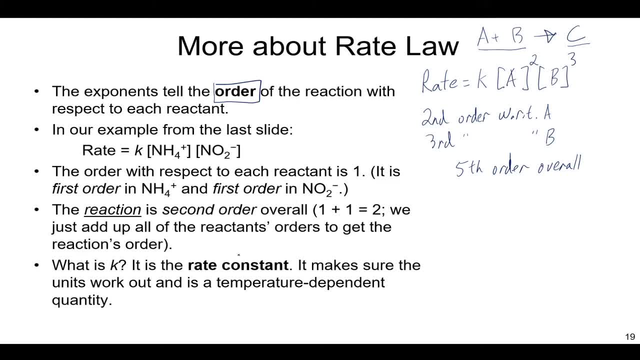 reaction orders. okay, as we've said before, k is the rate constant, it makes sure the units work out and it's temperature dependent. now, these orders- you just to drive the point home- must be determined experimentally. okay, this is super important, right? because the tendency is for people to look at. 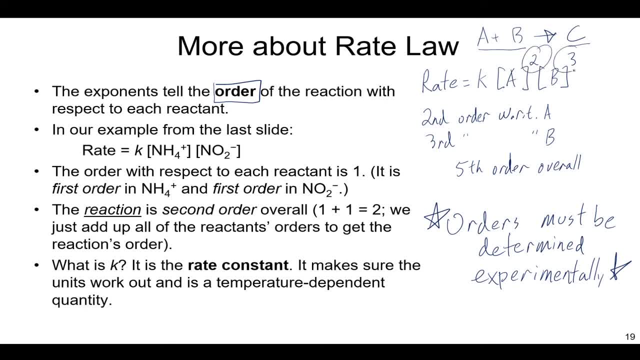 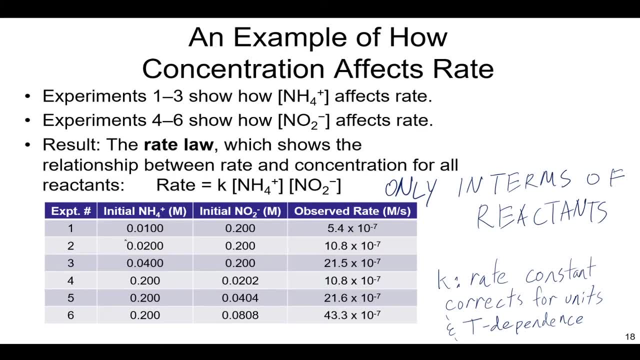 the overall reaction and guess at what the orders might be and derive a theory for how reactants turn out and how reactants turn out, and how reactants turn out and how reactants turn out into products. but you actually have to set up experiments. here's six different experiments: 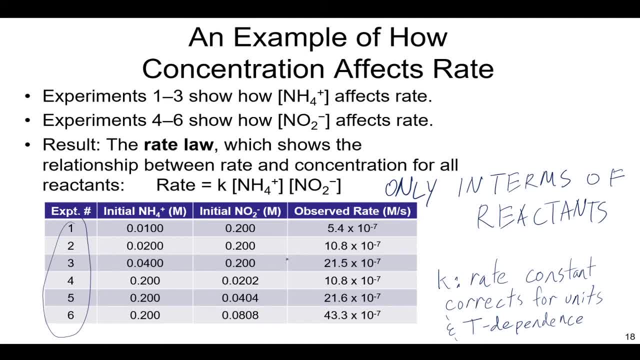 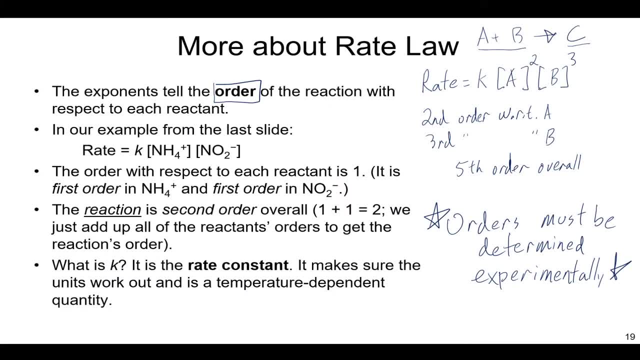 and follow these concentrations to determine what the observed rate is and thus the order with respect to each of these reactants. so that's really what we're after today: to understand how we would do such a thing. okay, so, uh, quickly, what i want to show you here, uh, in this table: 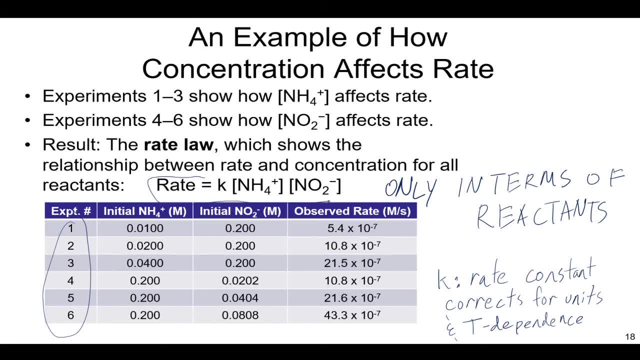 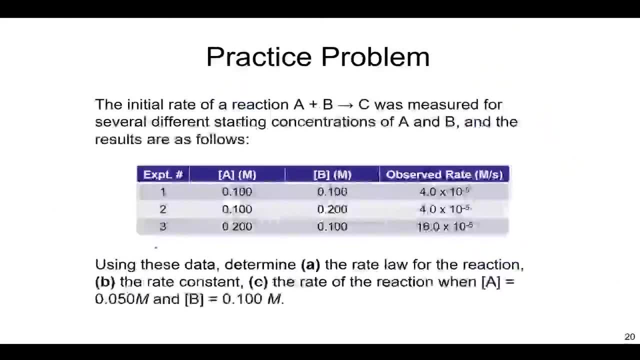 down table of data. how do we get this rate law? It's not given to us right? They're determined from experiments. So let's just look firsthand- And I don't think this is the practice problem, No- firsthand- at how we come up with this rate law. Right, And how we come up with this rate law is. 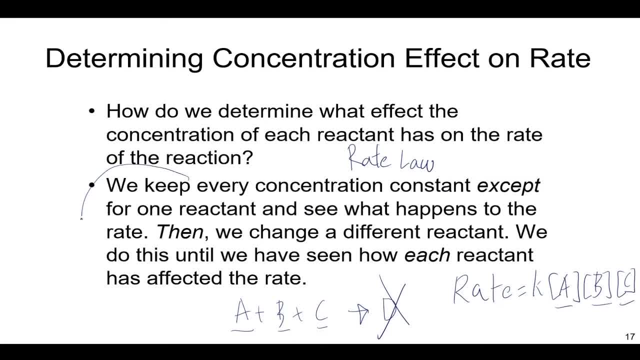 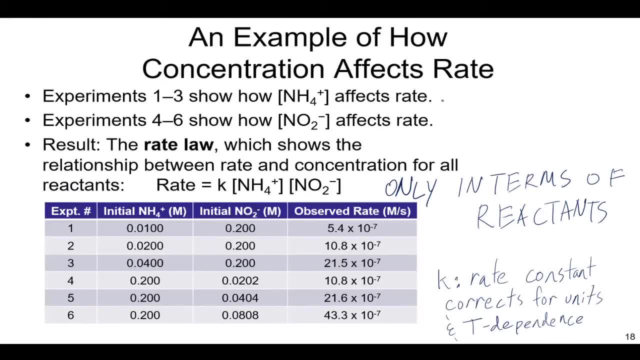 the following What we're going to do, as was suggested here, we keep every concentration constant except one of the reactants, and see what happens to the rate. So we know the rate law is going to look like. this rate equals a k times each reactant, And here the reactants are. 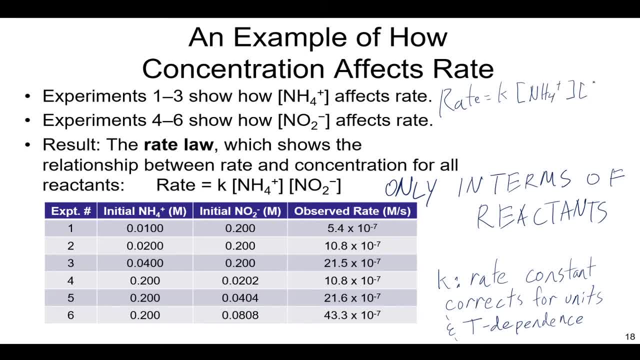 ammonium and nitrogen dioxide. But what we don't know, remember, is the order, So I'm going to put an x and a y here. Okay, this tells us their ones, but I'm giving you this for free. Let's see where. 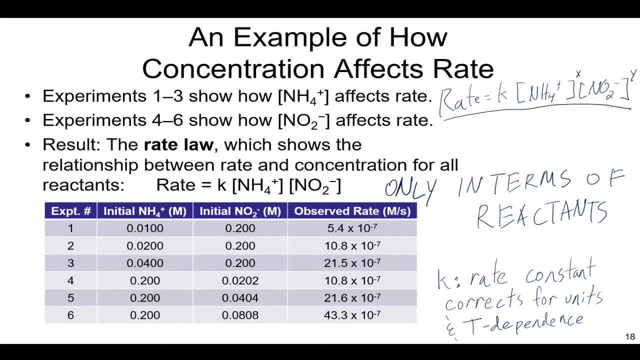 we come up with those ones from. I can immediately write this from the reaction. Okay, having told you that ammonium reactants are with nitrogen dioxide, right, you can immediately write the rate law as this, But now we have to determine x and y. the way we do that experimentally is to set up various experiments, So let's look at. 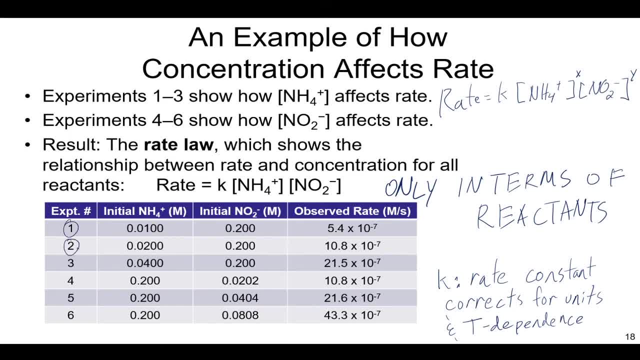 something. let's just look and compare experiment one and two And really here we have more experiments than we need. We really probably only need three here, But we can look at a couple of these one and two. no, two is constant, not changing, So whatever happens to the rate here. 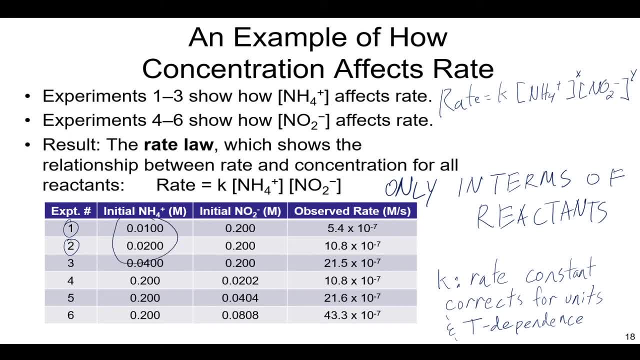 is solely determined by this change. So how we actually do this is what we put in a Beaker: this much NH for this much on code two. okay, we pour them in and we watched how NH four disappears in time. we catalog the time. we catalog the change in concentration. we divide. 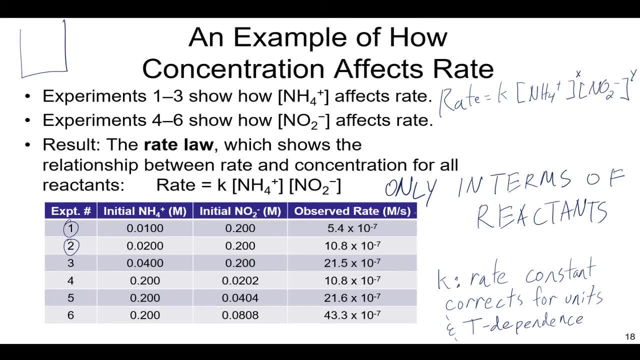 those things out to get our concentration per time, our observed rate. we did lots of those calculations in the previous video. Okay, so here we set this experiment one up. we get this data, we set up data. Okay so here we set this experiment one up. we get this data. we set up this experiment one up. we get this data. we set up this. 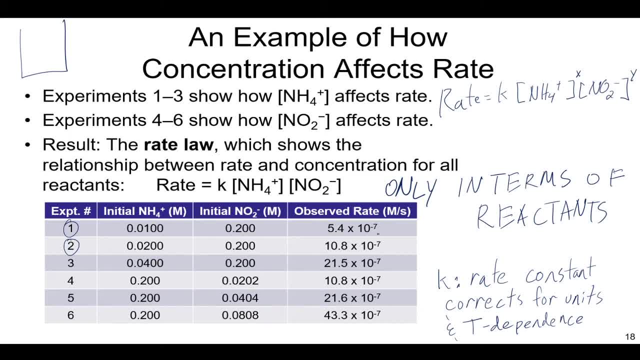 set experiment two up. we get this data. now we can compare the observed rate. okay, big number over the small number. 10.8 over 5.4 is two. so the reaction experiment two is twice as fast as experiment one. so the rate has doubled and this tells us. since i held no2 constant, since the rate constant isn't, 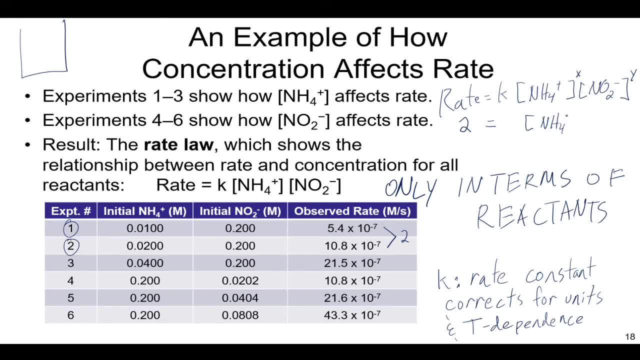 changing. this tells me the dependence on nh4 plus, because that's the thing i changed. so really, all you have to figure out here is: you know, two, what happened to nh4? it doubled. two is two. to what power, i wonder. i wonder if i can solve this. x is one, okay, so that's where the one comes from. 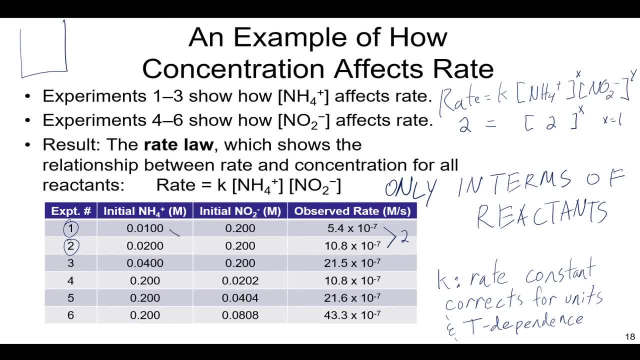 you plug in the data overall, you see the rate doubles when this doubles. so it's first order. so let's do the same thing, but instead pick two experiments where no2 changes, right, but nh4 does not, okay. well, that's easy enough, we can pick four and five. 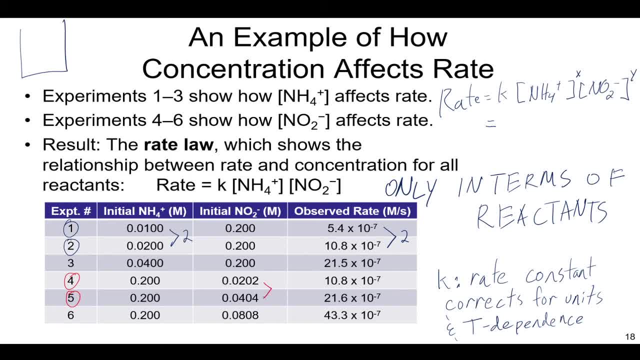 and four and five. nh4 is not changing, but any two minus is. this is doubling. and what happens to the rate? it doubles. so it's the same thing. the rate is doubling while no2 minus is doubling. i don't have to worry about nh4, i don't have to worry about the k, that'll. 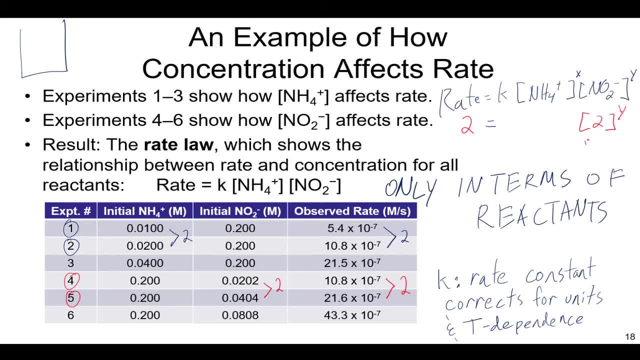 cancel out. so two to the y is two. well, y is one. so that's how i knew in the end that these were both ones and we don't have to write the ones. there we go. so that's how we go through and determine this. let's actually put it to work here in this practice problem. 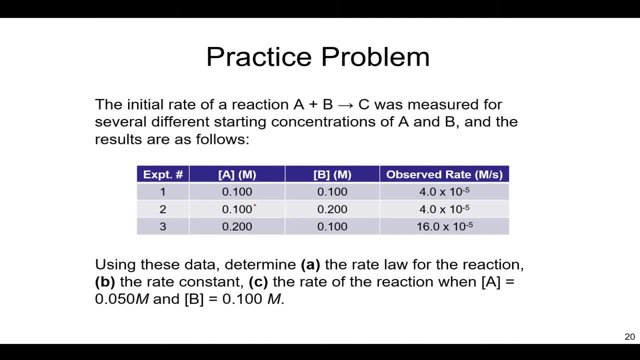 and use this data to determine the rate law, as i just showed you how to do it: the rate constant and the rate of the reaction for this last set of conditions. okay, feel free to pause the video here and try it yourself before i go through and solve it. okay, so immediately seeing this, 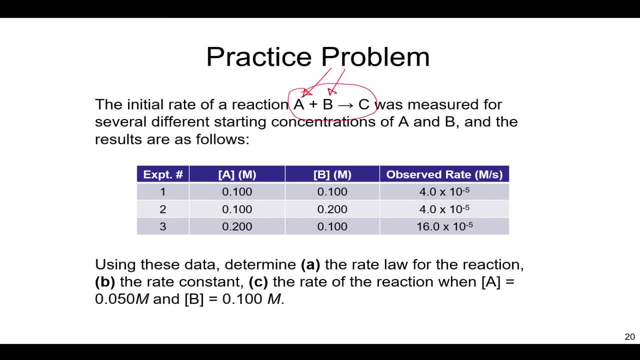 i'm going to just concentrate on the reactants. right, and i'm just concentrating on the reactants because i know the rate law just depends on the reactants. so rate equals k, concentration of first reactants to x, concentration of second reactant to y. so now let's go to the data and look. maybe we'll look at experiments one and two. 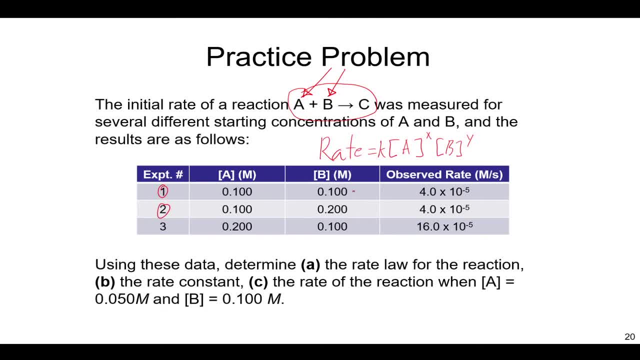 i'm going to choose those because one stays the same and b doubles. so from that data i can say what happens to the rate. the rate stays the same. it doesn't double, it stays the same. so i'll write a, one for the rate k. i'm ignoring a. i'm ignoring. 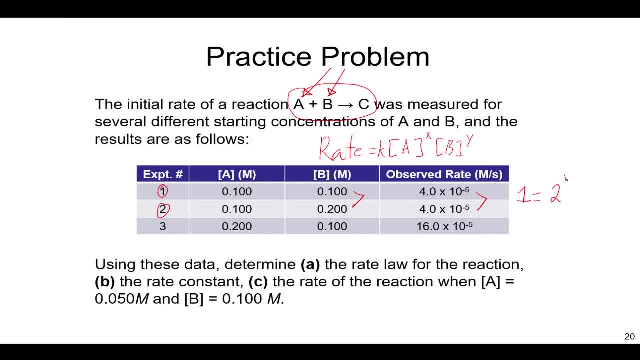 because it's constant, b doubles. so this is the equation i have two. to what power equals one? well, y here has to be zero. again, i picked two experiments where one of the reactants stayed constant, the other changed, and that will tell me the order. with respect to b, i double b. 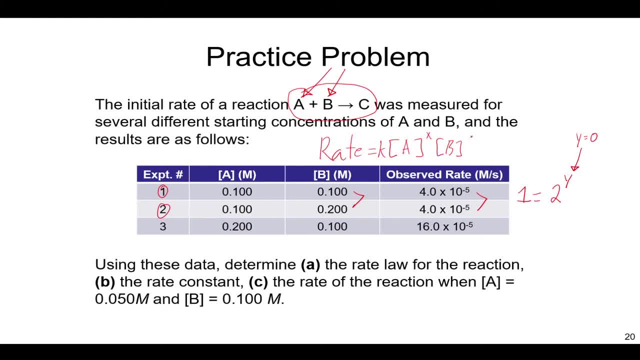 nothing happens to the rate. so the overall reaction is zeroth order. it does not depend on b. anything to the zero is one. so that's not part of the overall rate law. we can do the same thing, but try to determine a. and for determining a, well, i'm going to pick. 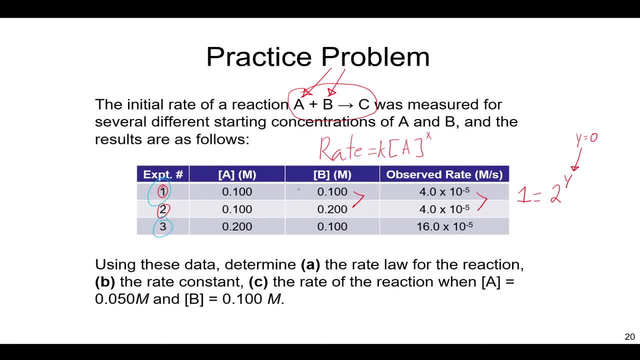 two experiments, one and three, and i'm going to pick those two because that's where b stays the same, but a changes, and that'll let me tease out the effect of a. so let's look at one and three. okay, three sixteen divided by four is four. so four is the effect on rate and four equals this doubles. 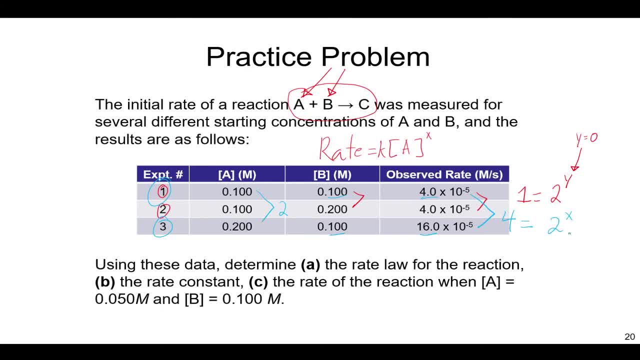 two to the power of x. two to what power is four? well, x, here is two, and that's how we figure out the overall rate law. okay, so our rate law here for this practice problem is: rate equals k times a to the second power, and that's our overall rate law. that is part a. so the answer to part a is rate equals k. 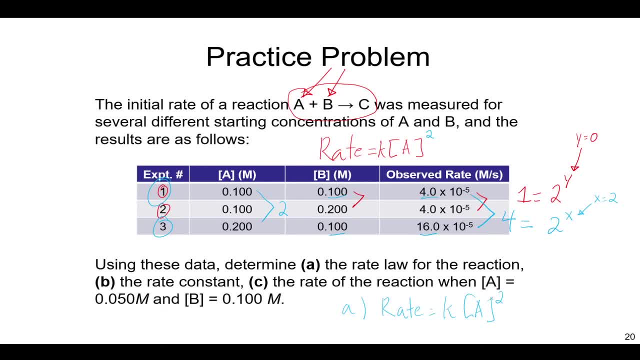 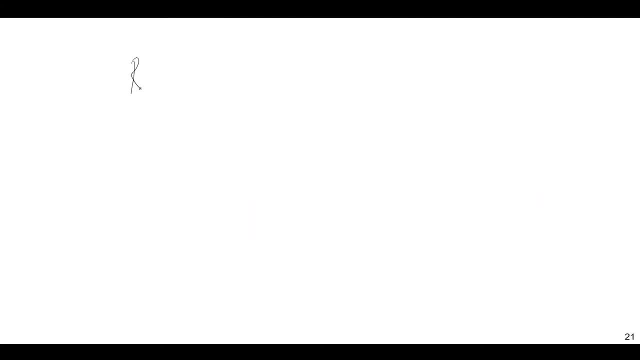 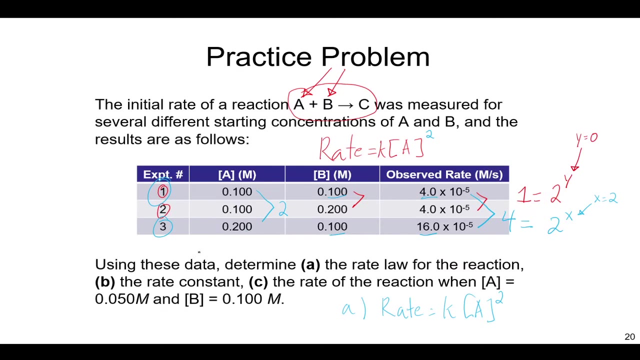 concentration of a squared. okay, it's second order with respect to a and it's zeroth order with respect to b. now for part b of the problem. what is the rate constant? rate equals k a squared in part b. i want to figure out the rate constant, and what's nice is now i have an equation. 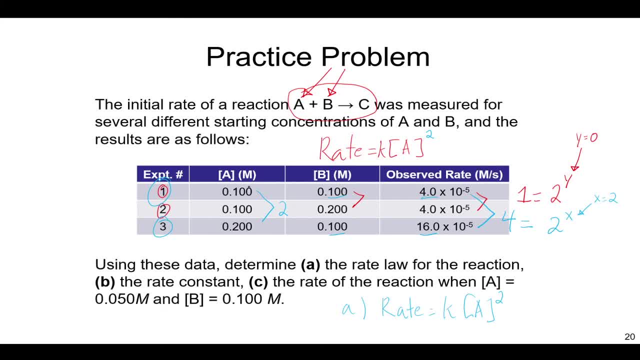 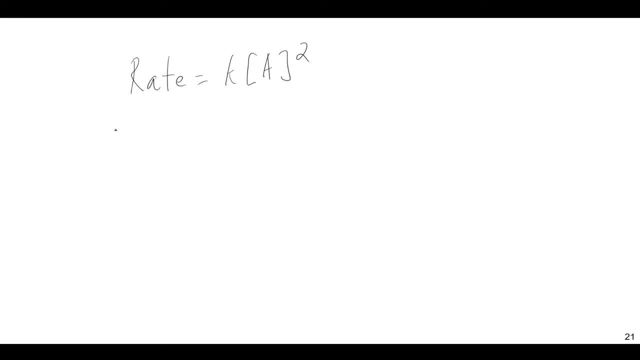 for the rate law. i can pick any single one of these reactions doesn't matter, and plug it into the rate law. so let me plug the first experiment into the rate law. four point zero times ten to the negative five equals k a, and the first reaction is point one: zero, zero squared. so 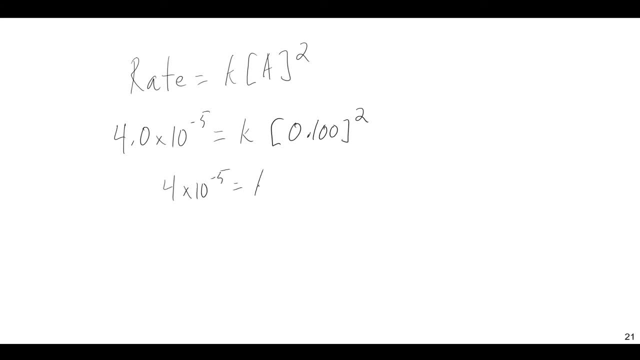 so four times ten to the negative five is k times 0.01 and in the end, the k value is going to be 4.0 times 10 to the negative 3.. okay, and that'll be my rate constant for part b. however, make sure you don't make this mistake. 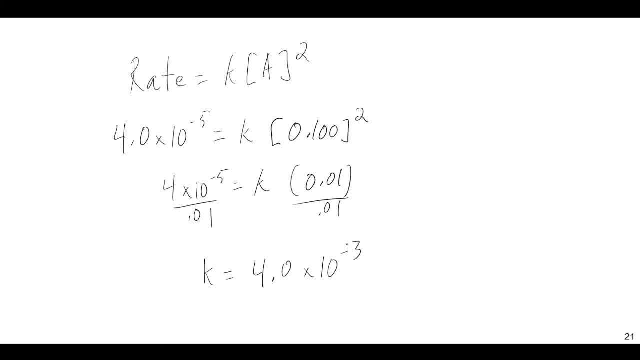 always include your units here on the rate constant and the units can get a little bit confusing. but realize that overall the rate is always molarity per second and the concentration here is molarity and that's squared. so that suggests that the units here for everything to work out, the units of k, is molarity. 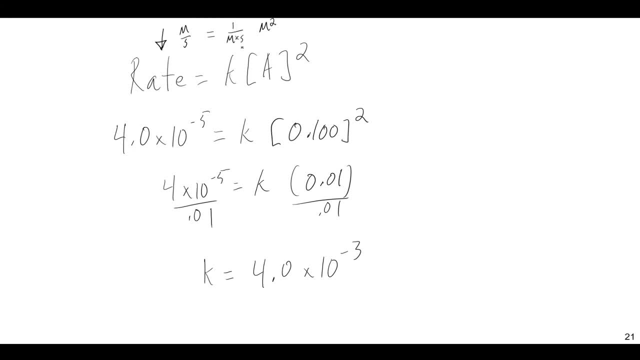 times seconds. that'll ensure that one of these polarities cancels and i'm left with the rate units of molarity per second. so here the rate constant units have to be four times 10 to the negative three, with the units one over molarity times seconds, or sometimes. 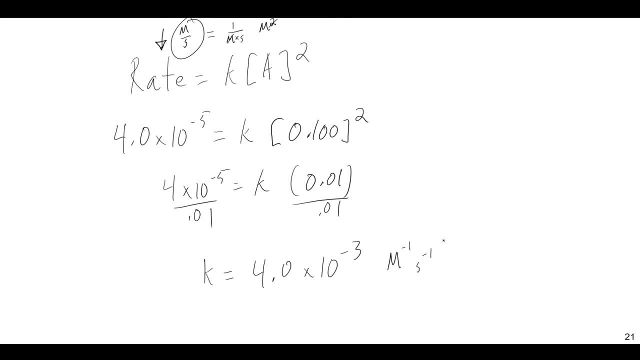 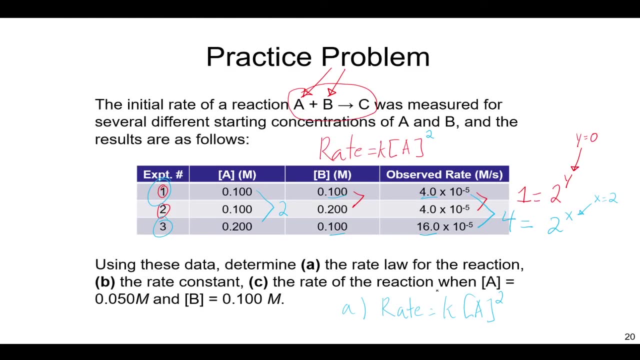 you'll see this written as molarity to the negative one, second to the negative one. okay, and so that's your part b, your part c here, the rate of the reaction when a equals 0.5 and b equals 0.1. well, we have k, we have an, a value. we plug them in again to the overall rate law. 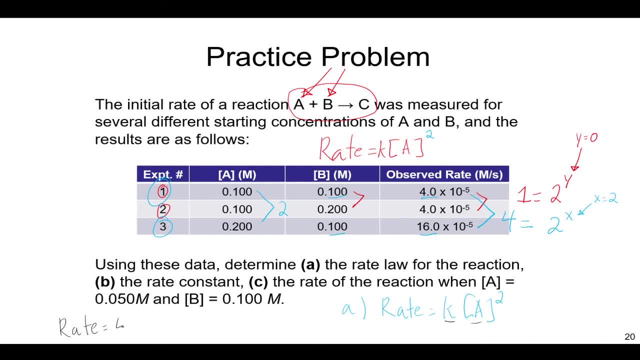 and the rate is going to be the k value. we just figured out 4.0 times 10 to the negative three over molarity, over seconds, times the concentration of a and part c. we're given 0.050 molarity squared, and now we solve for a or we solve for the rate, 0.05 squared times four overall then. 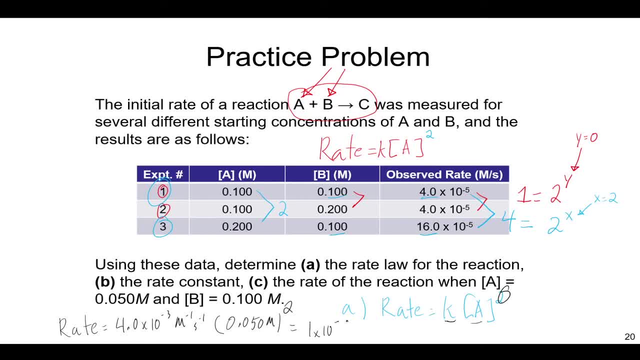 this gives us one times 10 to the negative five molarity per second. remember, the units of rate here should always be molarity per second. so that's our answer for part c. okay, so this is how we actually use experiments to figure out the rate laws. and this i mean can. 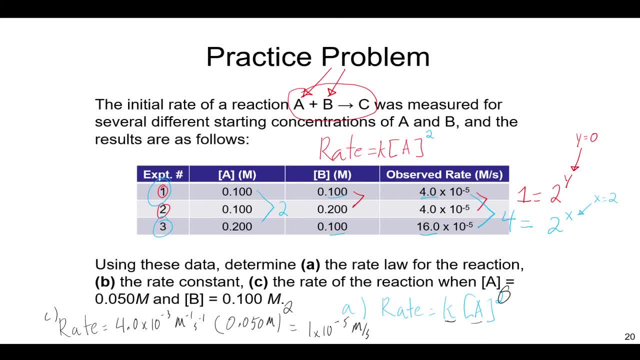 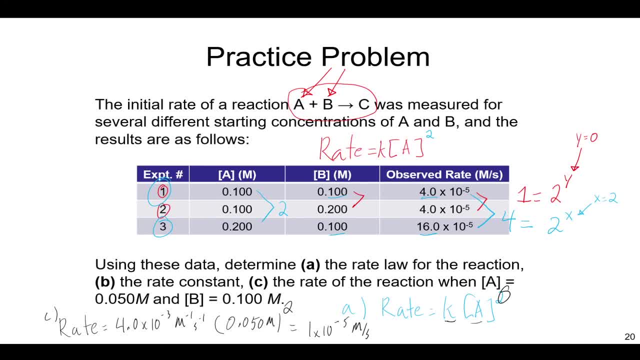 and how, how you can find half of it and how you can, depending on what you do- to be able to solve these quantitatively- is appreciate what this really means. okay, and what this really means is if i'm trying to create a drug right that targets 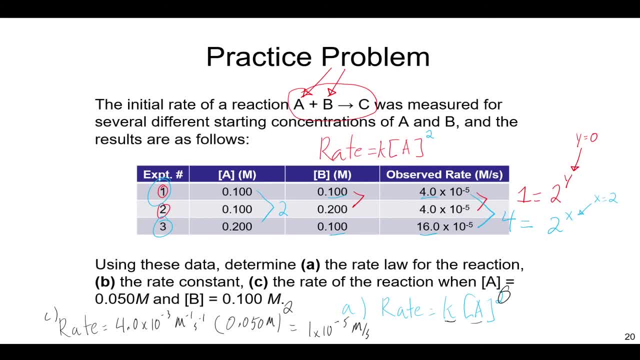 some active site of an enzyme, the way i figure out what is the mechanism for the reaction that i am trying to inhibit. okay, i figure that out by mixing up amounts of the active biological molecule, amounts of the enzyme and figuring out from a bunch of different concentrations. 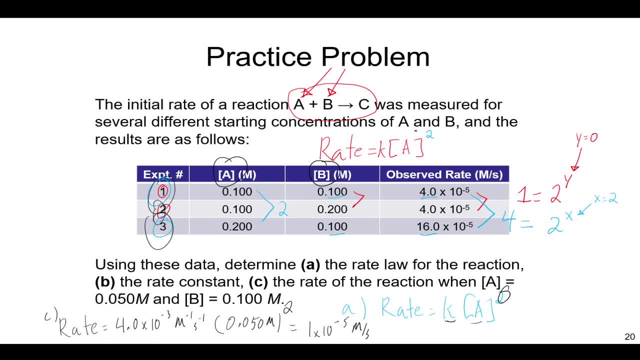 and a bunch of different experiments here. what is the rate law for the reaction? I care about, And once I know the rate law for the reaction, I care about this two, as we'll see in future lectures. this two right here tells me: